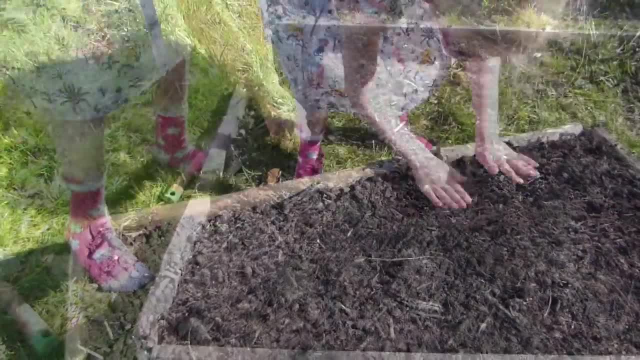 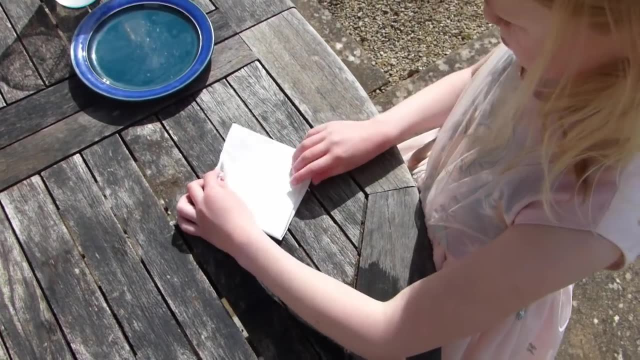 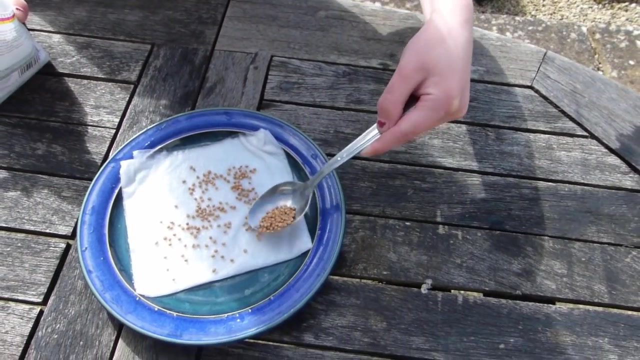 so that they have a real sense of ownership over their space. This is absolutely the best way to keep them excited and engaged with the whole process. If you don't have a garden, sow something indoors. Sow microgreens such as cress or mustard onto damp paper towel. 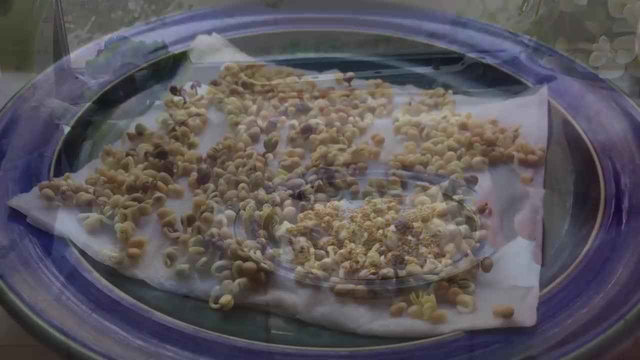 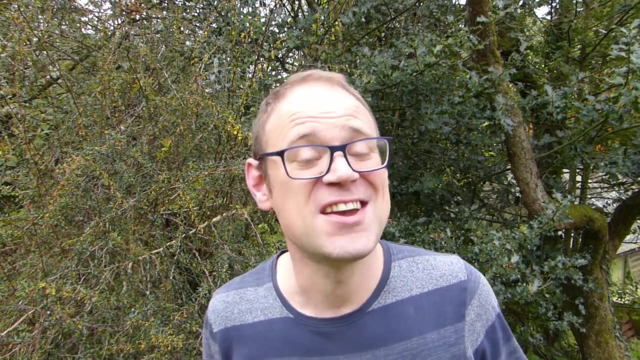 Move them to a bright window sill once they've sprouted and keep them damp. They'll give something tasty to eat within a matter of days. How about a little biology? Teach your children how germination works by sprouting bean seeds in a jar like this. 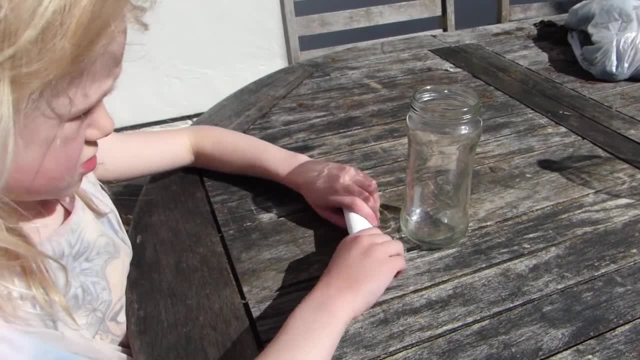 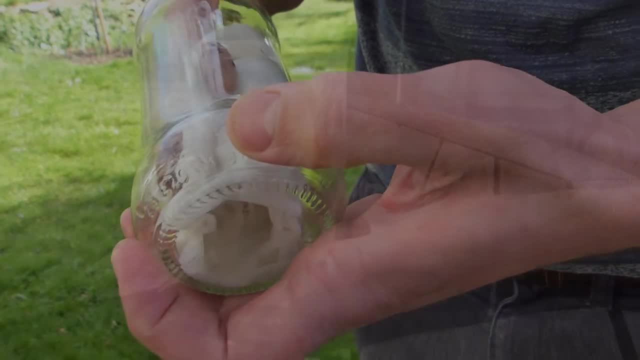 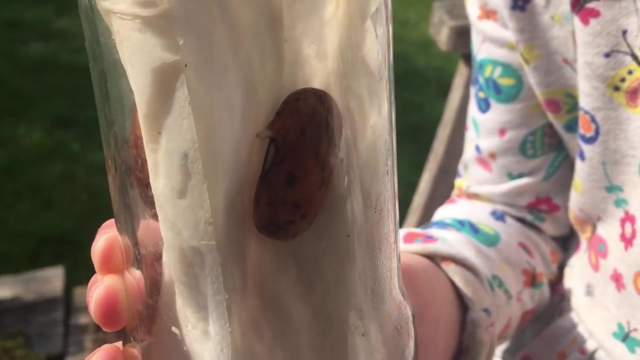 Roll up several sheets of paper towel into a cylinder then pop them inside a clear, clean jar. Dampen the paper, then push some bean seeds that were soaked overnight in between the glass and the damp paper towel. Check regularly for signs of germination and observe the roots and shoots as they push through. 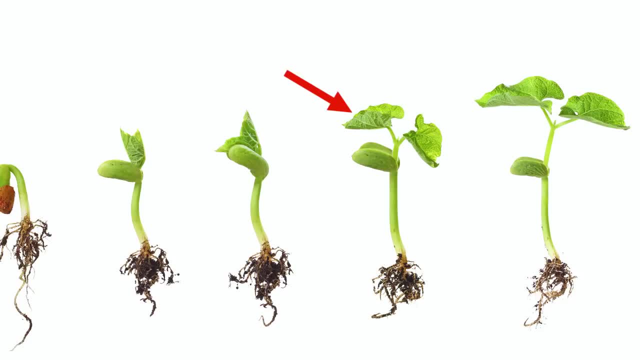 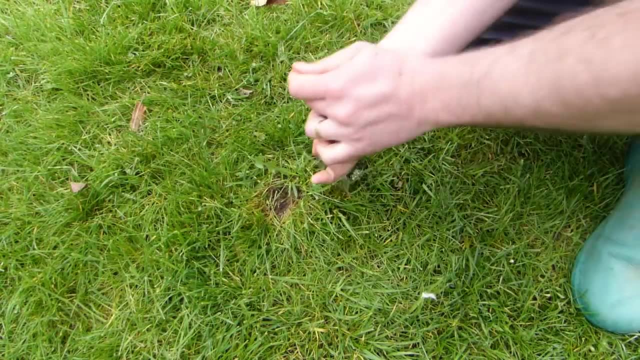 Explain the difference between the young seedling leaves and the first true or adult leaves. Another fun project is to dig up and pot on a young dandelion. Dig up as much of the long taproot as you can and transplant it into a container of soil or potting mix. 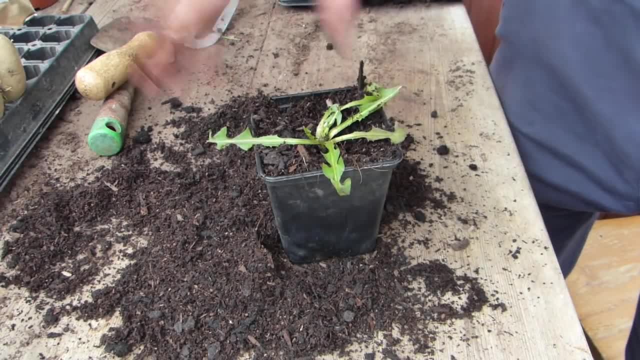 Give it a water, then move to a window sill. Rather than being mown or cut down, you can also plant it into a container of soil or potting mix. If you're weeded out this way, they'll get to see how the plant produces its flowers and seeds. 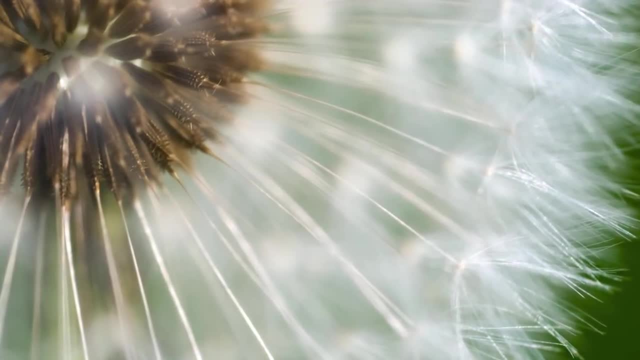 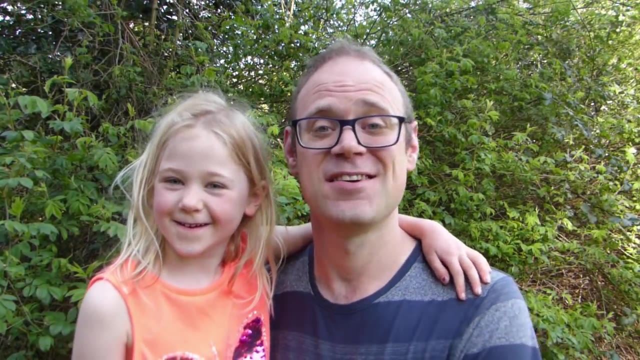 Why does it do this? Can they guess how many seeds there are and how would the seeds get dispersed? Send them out into the garden to look for bugs. How many can they find? What was it you found last week, Isla? 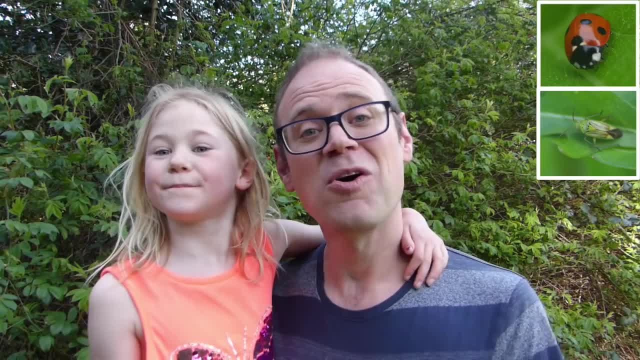 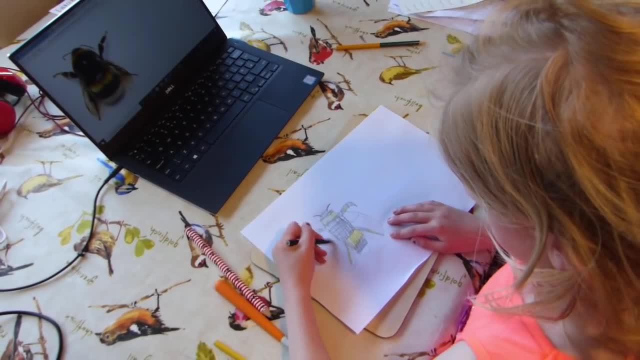 A ladybird and a green shield bug. What can your little ones find? Help them report what they found on the Big Bug Hunt website. If they're feeling arty, send them to draw their favourite bug: Isla's having a go at a bumblebee. 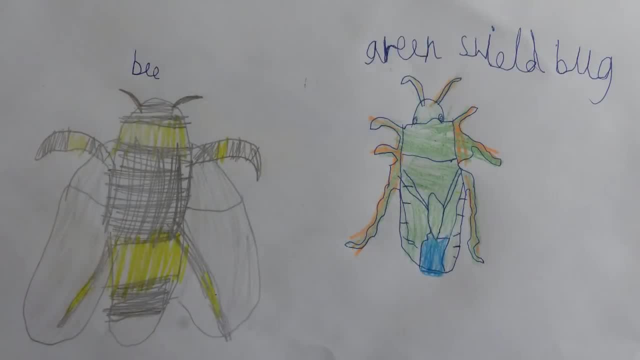 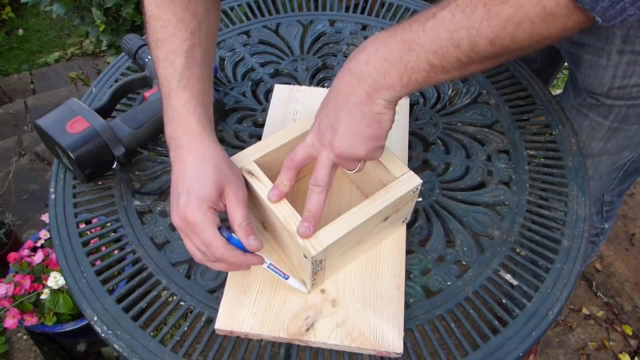 Try drawing from memory, or use a photo as a guide. Don't forget to colour it all in. Hey, and don't forget to look after our six- and eight-legged friends as well. Try making a bug hotel. Find out how to do this in the video description below. 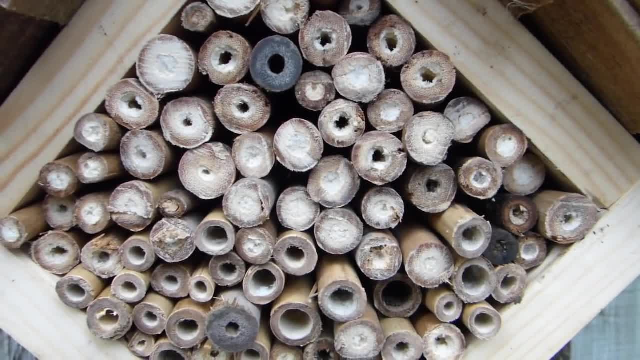 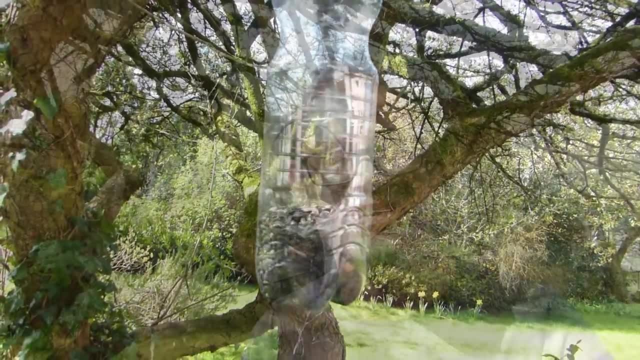 It's a really fun project and you can use scraps from around the garden to fill it. Or how about this swanky bird feeder? It's very easy to make. All they will need is a plastic drink bottle or milk jug, some scissors. 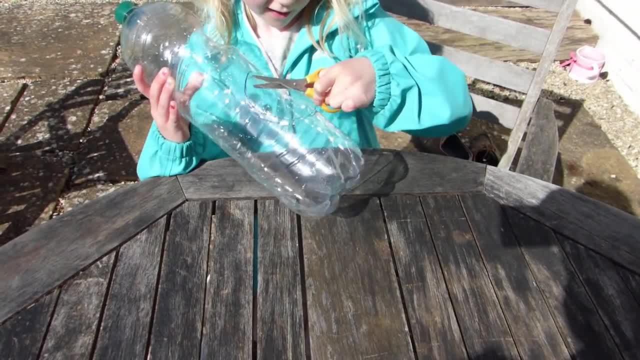 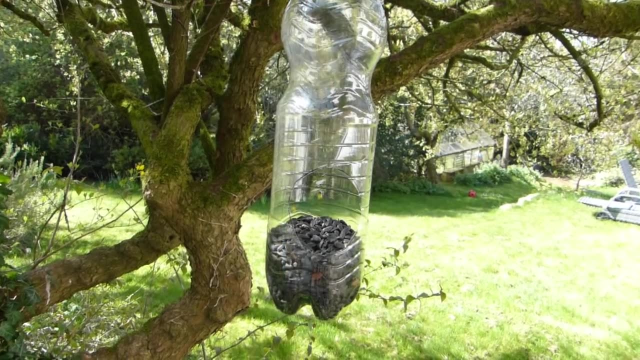 and some string to hang it up. Begin by getting them to cut out a hole in the bottle, roughly 3 inches from the bottom. The hole needs to be circular or oval in shape and about 3 inches wide. Now poke holes into the bottom of the bottle. 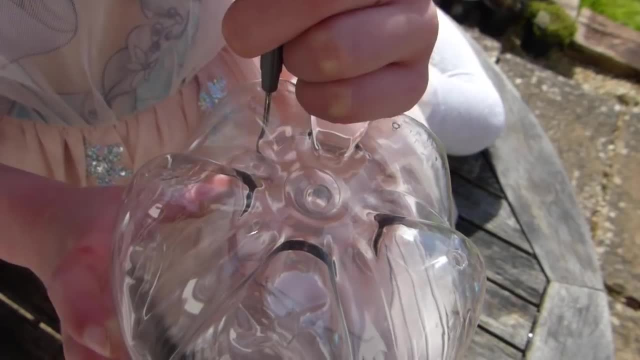 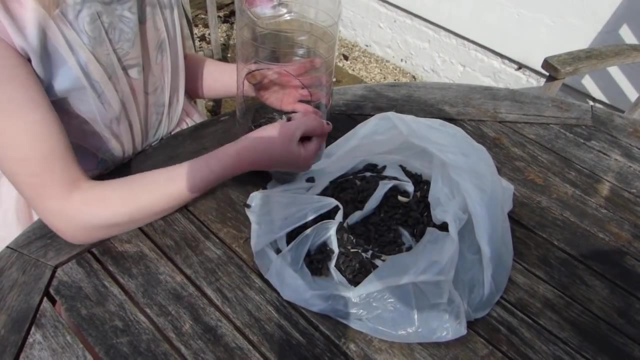 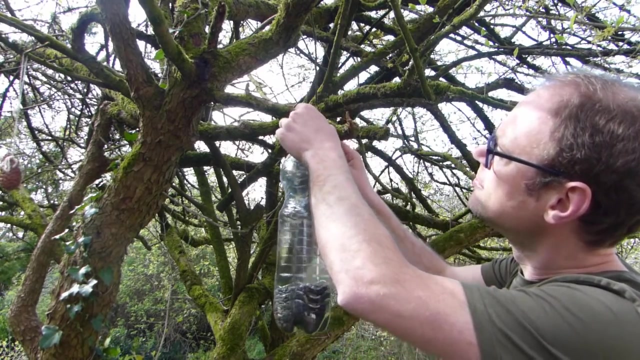 so that any rain that gets in will be able to drain away. It goes without saying that young children will need to be supervised. Attach the string to the top of the bottle and fill the feeder with birdseed or nuts. Hang the feeder up in a tree off the ground so it's clear of the neighbourhood cats. 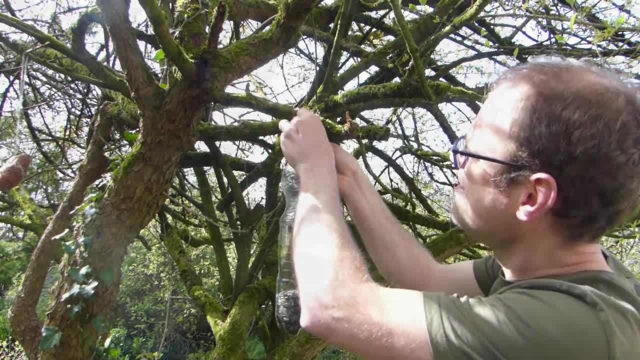 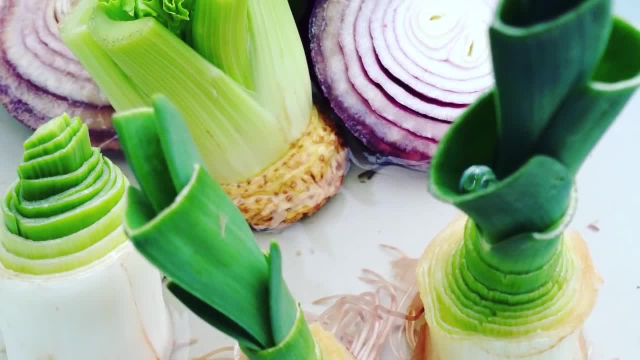 Now get them to record what birds pay a visit. With any luck, it'll keep them amused for hours. Did you know that many kitchen scraps will sprout into new plants if given a little water? This includes the tops of carrots, beets, pineapple and turnip. 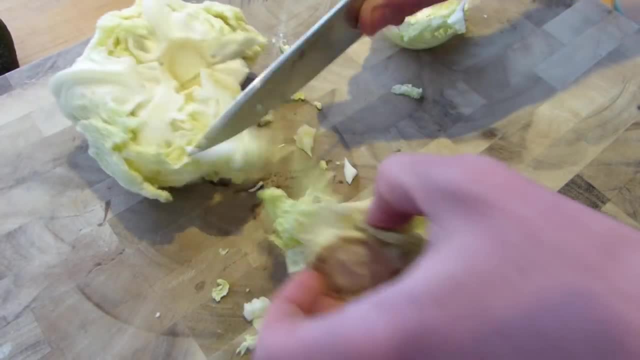 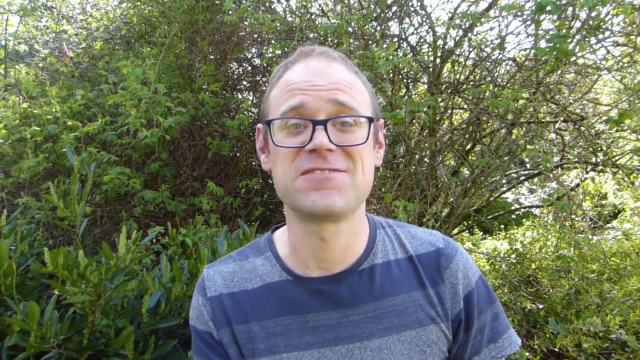 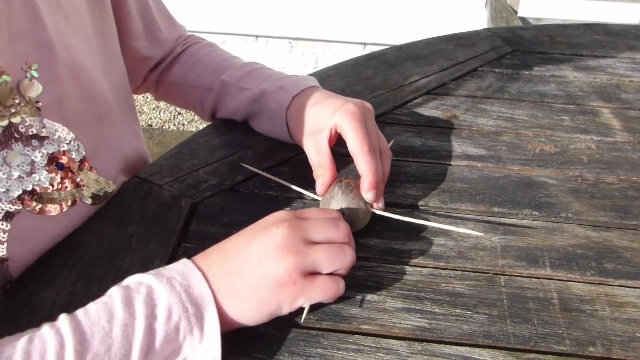 as well as the stumps of vegetables like celery, lettuce and onions. Sit them in a saucer of water and watch them burst back into life. Another very satisfying project is to sprout an avocado stone. Take a washed stone, then push in 3-4 toothpicks around the middle of the stone like this: 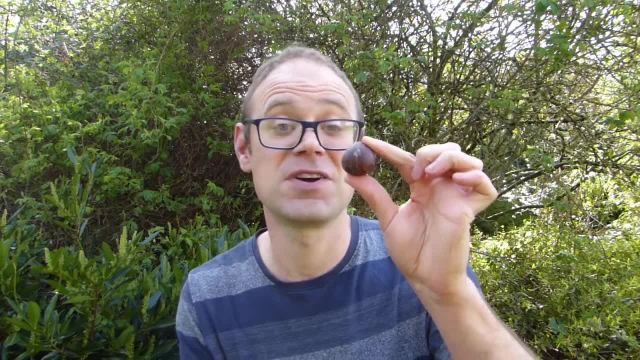 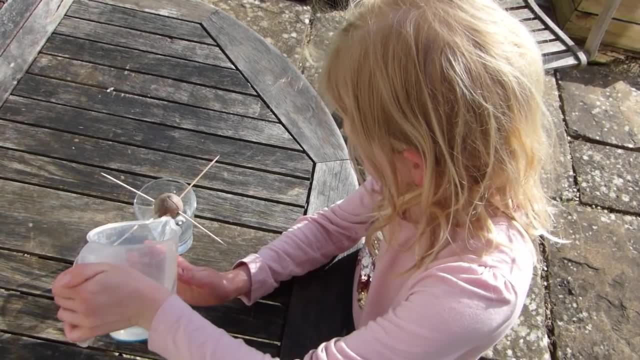 You want the pointiest end of the stone to face upwards, because this is where the shoots will sprout from Now, use the toothpicks to rest the stone on a glass jar. Top it up with water so the water reaches the bottom of the stone. 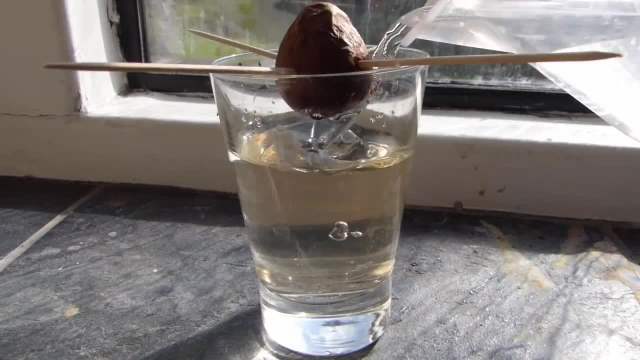 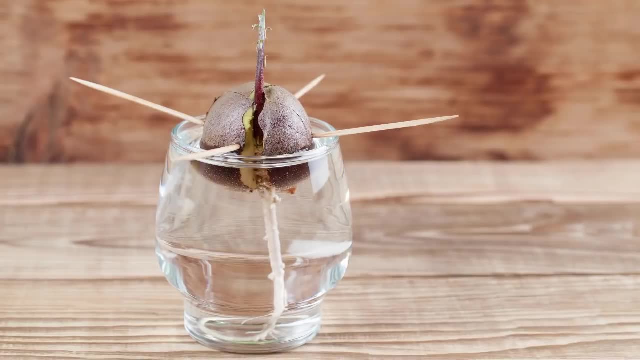 then pop it onto a warm, bright window sill. Top up the water every now and then, so the bottom of the stone remains covered. The stone will sprout within one to two weeks. Once it has grown into a sturdy seedling, transplant it into a container of potting mix. 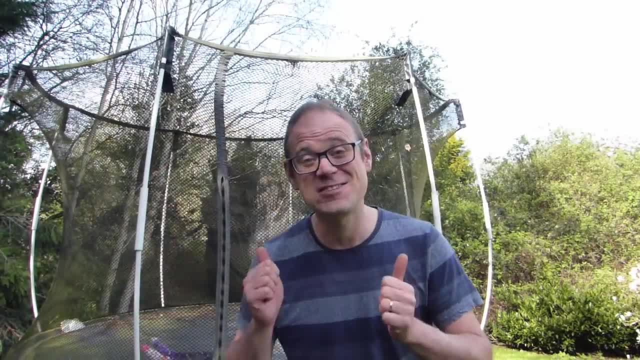 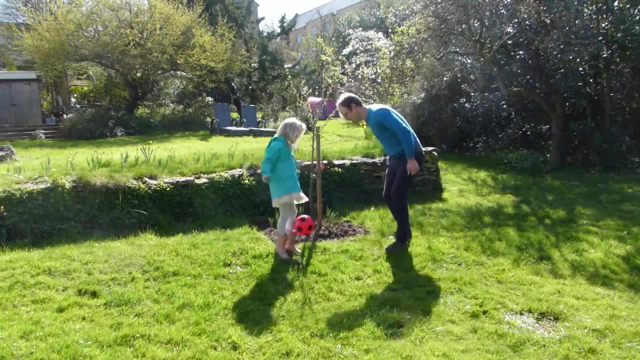 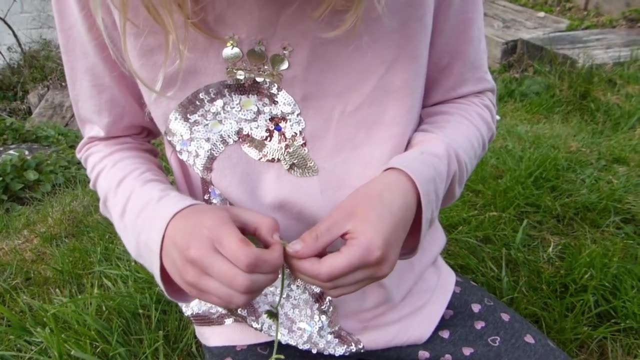 Exercising outdoors is beneficial for everyone, especially children. Get them jumping, bouncing, running, kicking, whacking- anything to expend just a little fraction of their boundless energy. Revive some of the traditional childhood activities too. Daisy chains are always fun to make, though. save some flowers for the bees. 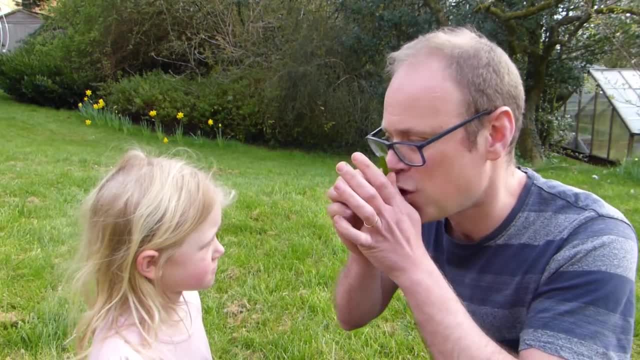 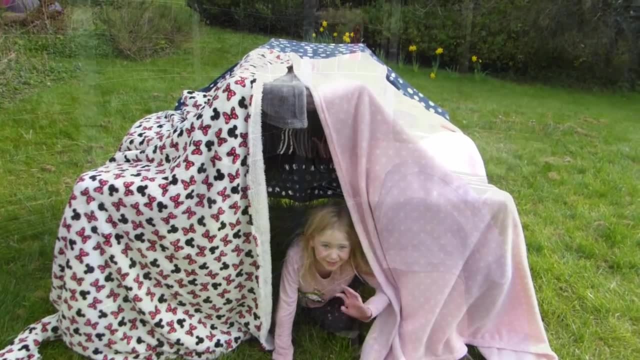 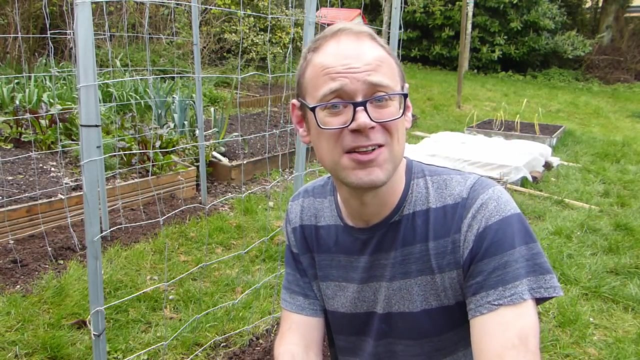 Use wide, long blades of grass to make a honking noise, Collect different flowers and leaves to press into an album, or build an outside den using blankets. That should keep them busy for a while. Don't forget the huge range of online resources as well, full of many inspirational ideas. 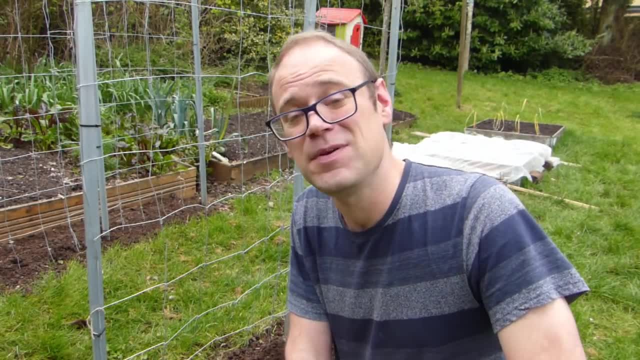 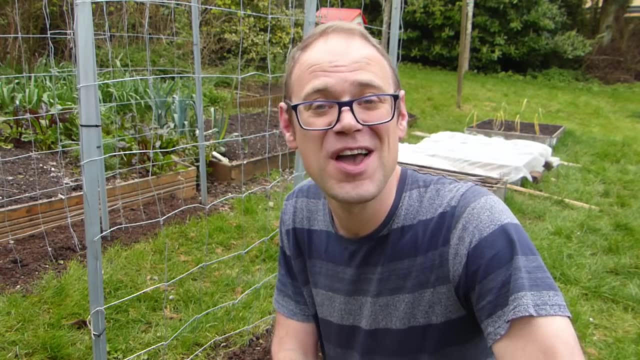 We've listed a few of them down below. Tell us how you're keeping your children amused during the lockdown. Is your garden proving to be a handy outdoor classroom? Share what you're up to in the comments section. It's great to have you watching. it really is. 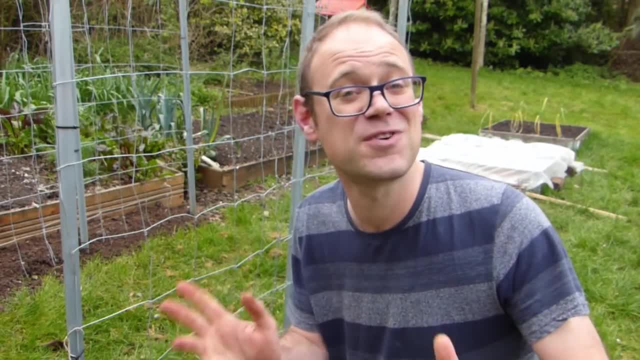 Please stay positive, keep happy and healthy and, of course, continue to enjoy your garden. I'll catch you next time. 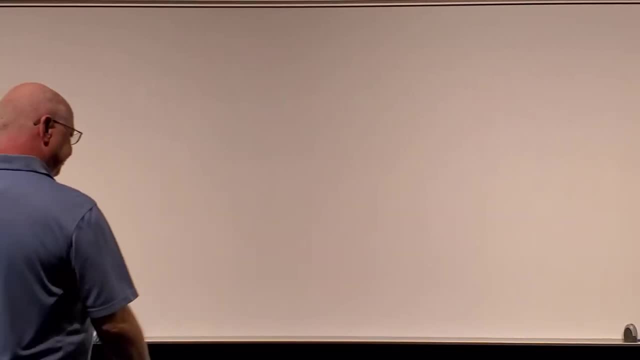 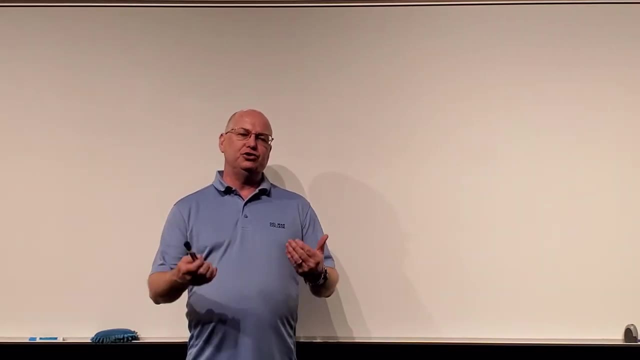 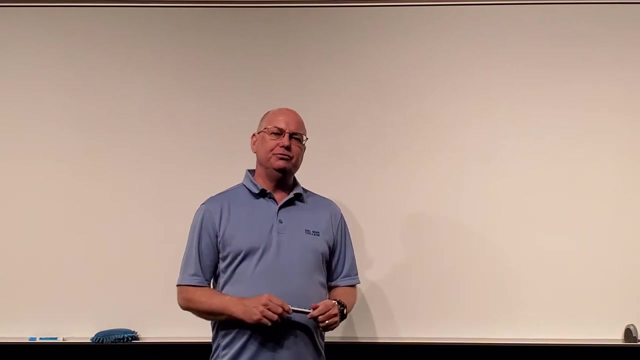 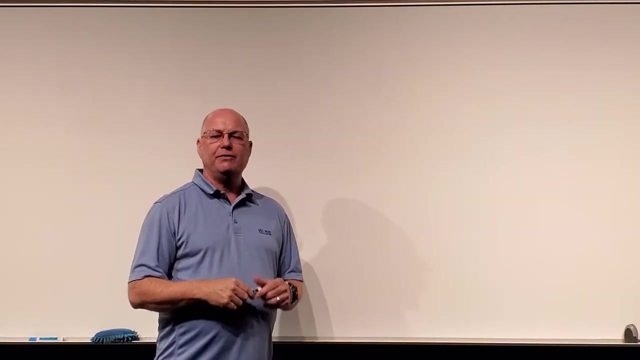 Hey everyone, welcome to Professor Long's Lectures in Microbiology. These videos are intended for use by students who are enrolled in My Biology 2420 or Microbiology for the Health Science courses at Delmar College. If anyone else out there in YouTube land finds them helpful, by all means please hit like, hit subscribe or provide me some feedback so that I learn how helpful they are for you and I can continue to do these videos if I'm encouraged to do so. 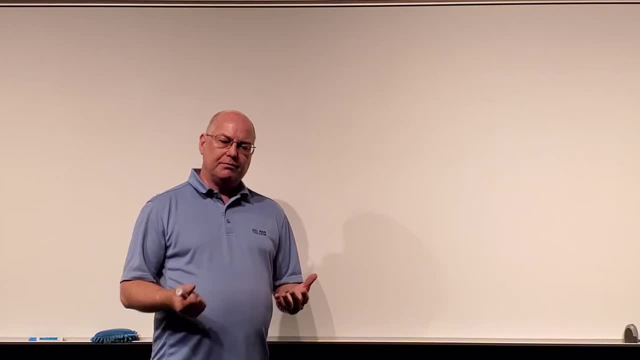 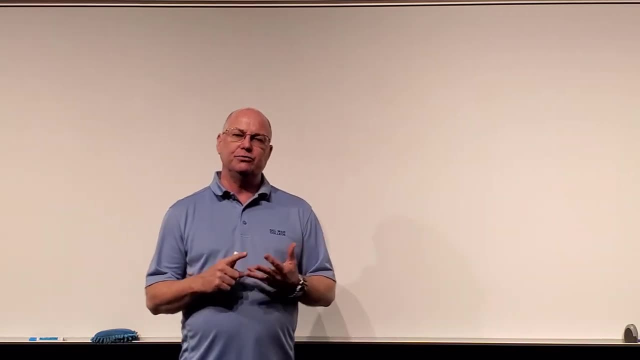 Now, when you take microbiology, we're going to get into chapter one, the introduction of microbiology. We're going to go a little bit over the history of microbiology and some terminology to set some of the basic foundation of this course. 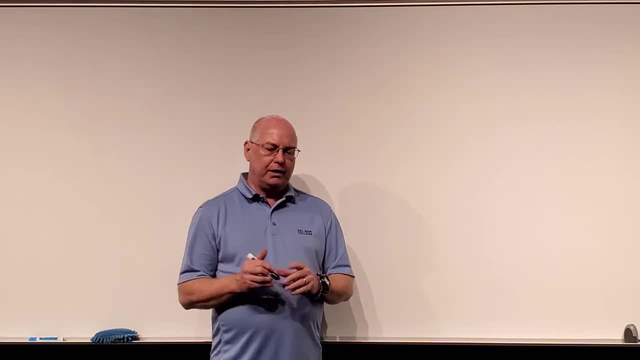 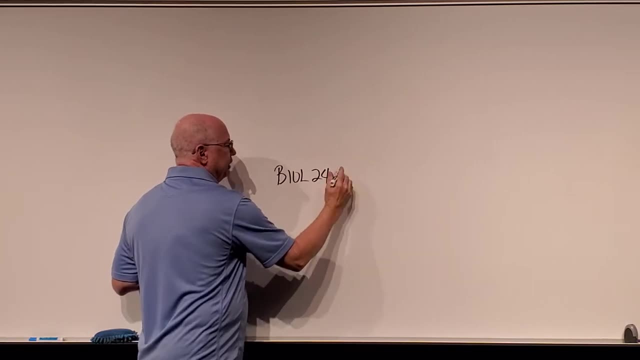 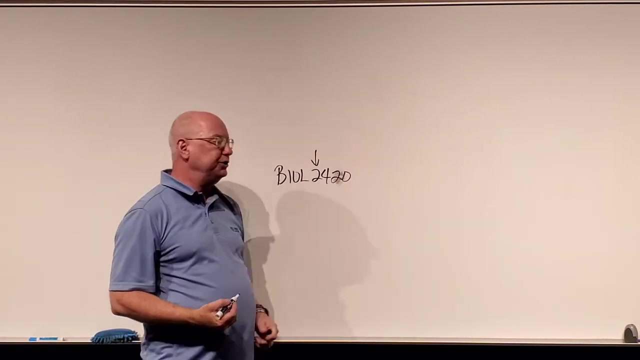 Now, typically, if you take microbiology, the course number throughout at least the state of Texas and most universities throughout the nation is 2420.. This number tells you it's a sophomore level course. So you have freshman, sophomore, junior, senior. This number tells you the number of hours we combine the lecture and the lab and there is a lab component for this course. 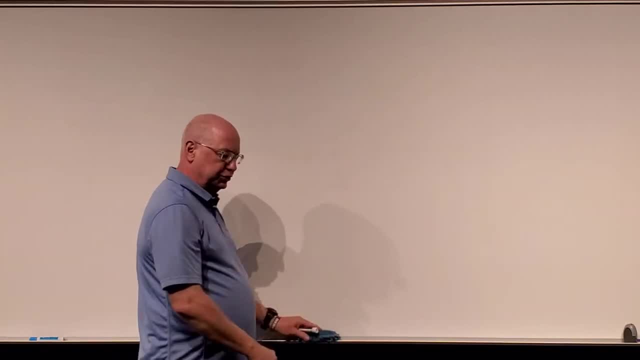 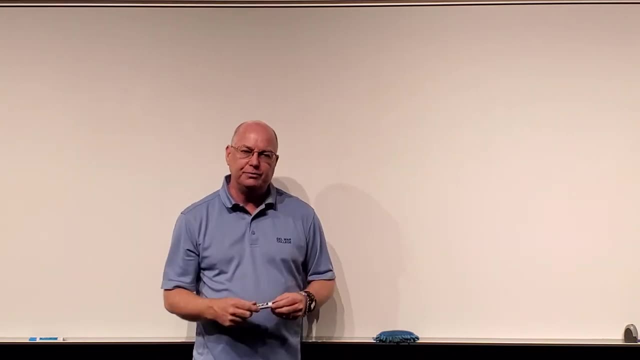 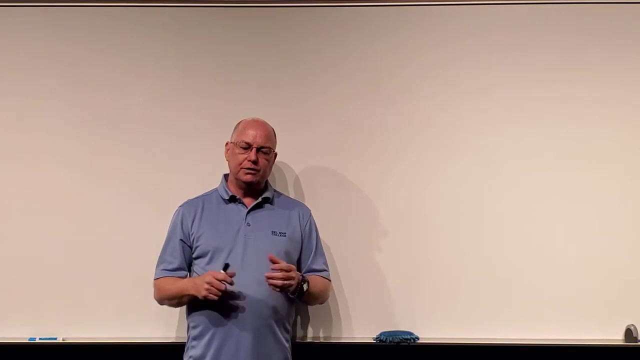 So this is a sophomore level biology course. Take sophomore level courses. you have to pass a certain number of freshman level courses, like Freshman Biology 1 and 2 and some Freshman Chemistry. Now, in their grand wisdom, the politicians that run things have decided that colleges are getting rich by making you take extra classes. They want you to hurry up and get out and start paying taxes, at least in my opinion- And so they have mandated that all associates degrees be cut to 60 hours and all bachelors degrees be cut to 180.. 120 hours. Well, the problem is, some degrees require a few extra courses. My biology degree.